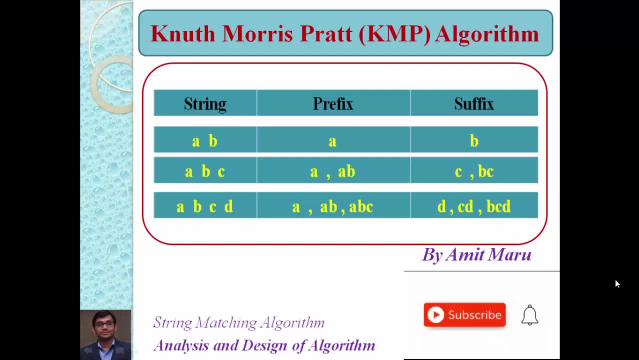 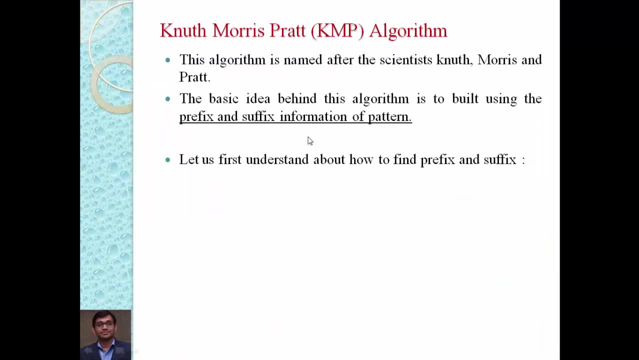 The basic idea behind this algorithm is to build using the prefix and suffix information of the pattern. So when we compare our pattern with the tags, at that time we are using prefix and suffix information and based on that we will compare our pattern with the tags, And this is the logic of KMP algorithm. So before starting of the KMP algorithm, 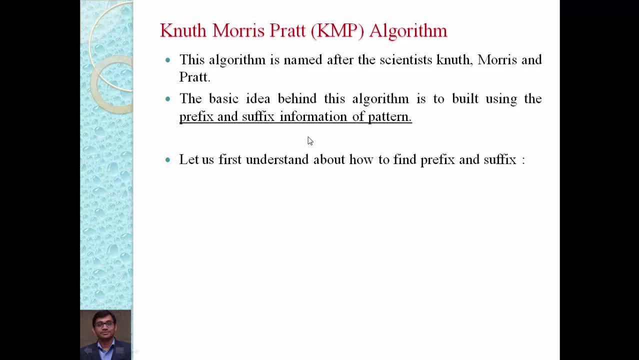 You must know how to find a prefix and suffix of any pattern or any string. So let us take a different example. Suppose our string is A and B. Our string has a two character, A and B. Then the prefix and suffix of A and B string is: A is before the B, so that the prefix is A, and B is after A, so that the suffix is B, If only two characters are there. 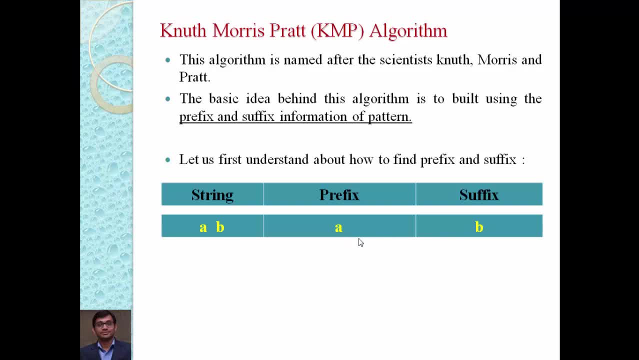 Then first character will be prefix and second will be suffix. but whenever three characters are there at that time, what is prefix and suffix? So the prefix of ABC is A and AB is the single character A and the pair of character AB. These both are the prefix because it is available before the C character. Now if you want to find the suffix then 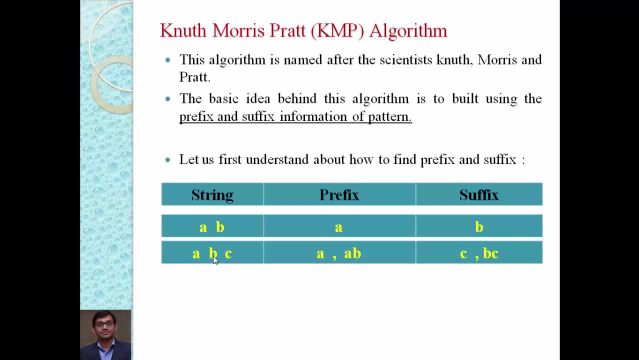 It must be after, so that after A We have 2 characters, character b and c. so we have to use for single character. single character is c, so c is a suffix and the pair of character b, c, it is also suffix. so the prefix is a and a, b and the suffix is c. 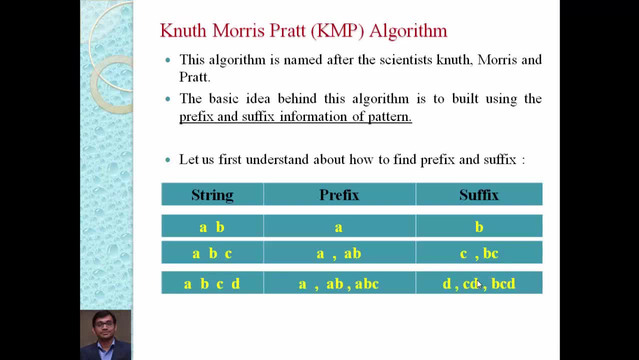 and b, c. if more than three character, or we can say four characters, are there, then we can say before d we have three character, a, b and c. so based on that we have to identify prefix. so prefix is single character a, then after pair of character a, b and three, pair of three character. 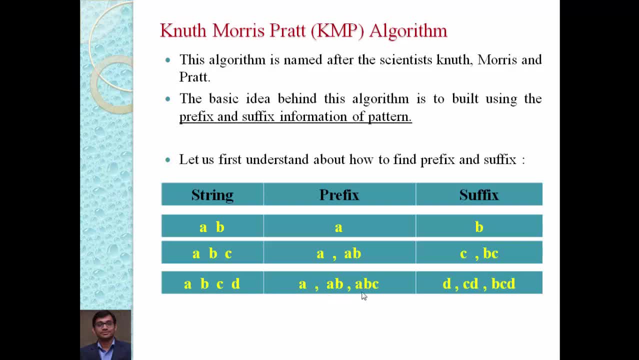 in a pair that is a, b and c. so these all are the different prefix and suffix of this: a, b, c, d is after a. we have a three character: b, c and d. see the single character d is a suffix pair of character c, d is a suffix and b, c, d is also suffix. 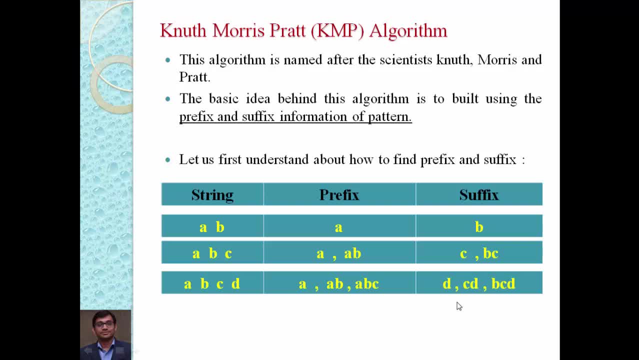 so in this way we have to identify prefix and suffix information of the pattern and this information is very important in our kmp algorithm to shift our pattern when we match our pattern with the tags. so let us understand first different steps of kmp algorithm. so now let us discuss. 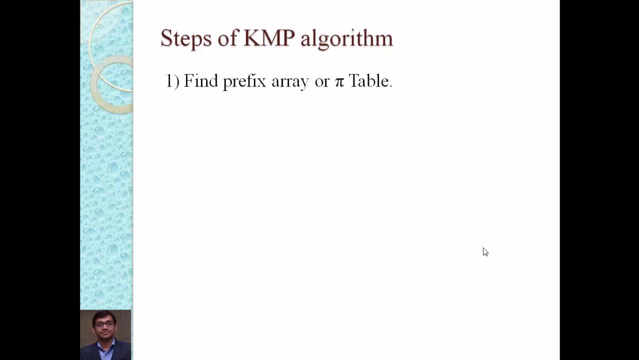 different steps of kmp algorithm. step number one: find out prefix array or pi table of the pattern. so we have a set of a character inside the text and some character inside the pattern. so the first step is we need to identify prefix array or pi table of the pattern. step: 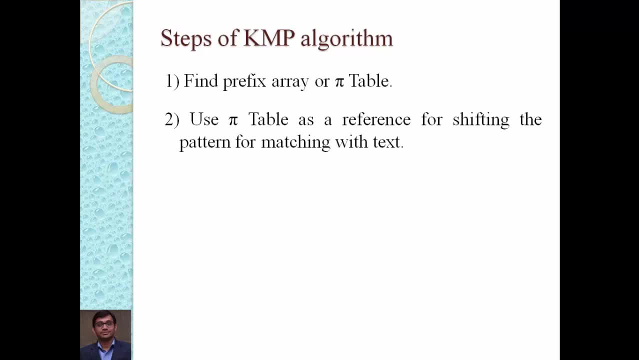 number two: use pi table as a reference for shifting the pattern, for matching with the text. when we compare our pattern with the text then we need to start from the location number zero or we can say zeroth index and as per the new method, we are just shifting our pattern by one, but here we are not shifting every time by one, but 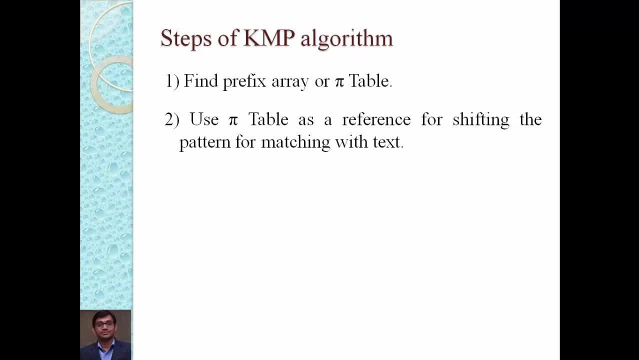 we have to use pi table as a reference to shift the pattern to match the character with the text. step number three: when all character of the pattern match with the text, use following formula to find out the index number. so formula is i minus length of pattern plus one will. 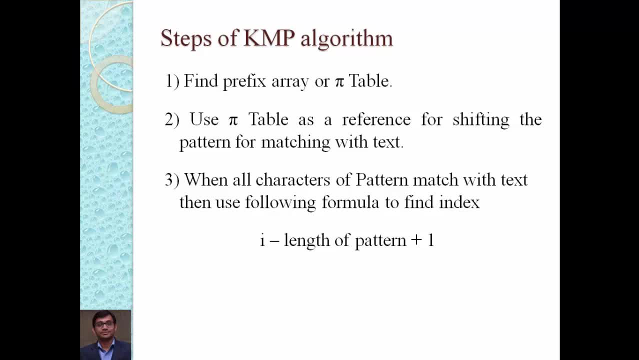 give us index number where our pattern is matched with the text. so these are the different three steps we need to follow when we apply our kmp algorithm to find the pattern inside the larger text. let us take one example in that we will use these three steps to find out. 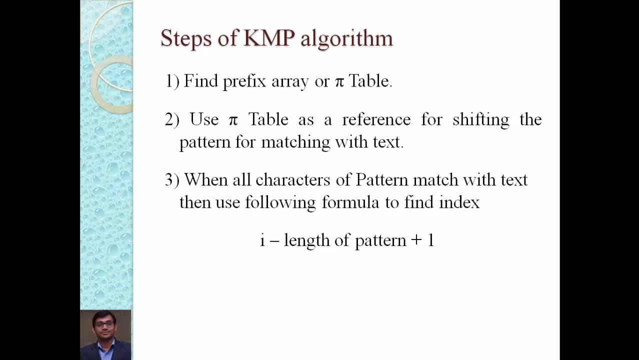 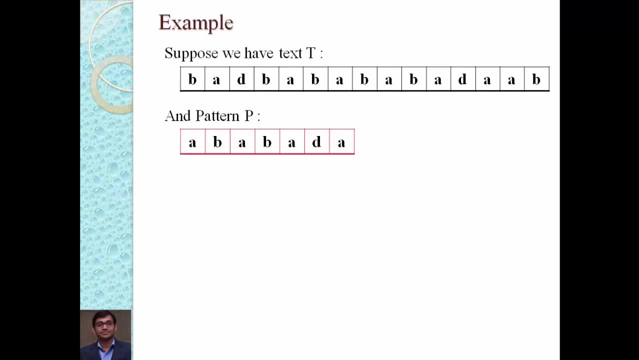 whether our text, whether our pattern, is available inside the large text or not. once it is available, then this last step will return index number. let's take one example. let's take one example in this example. suppose we have a large text, capital t, in that number of characters are. 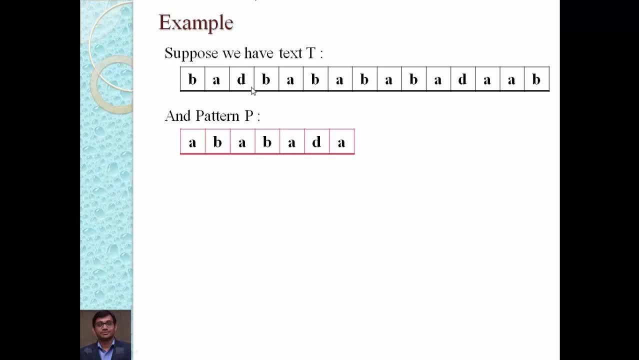 there and we have one pattern, capital P, which has some character here. total seven characters are there inside the pattern. now we need to identify whether this pattern is available in this text or not. if it is available, then we need to return the index number. so let us start. 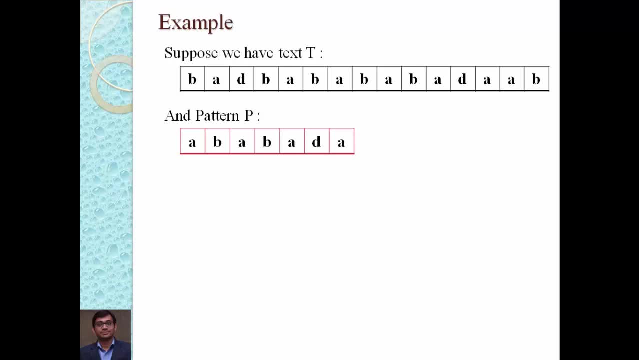 by using kmp algorithm. So, as per the KMP algorithm, our first step is: we need to identify prefix array or PI table of the pattern, Right? So let us find out PI table of the pattern. So, as per the first step, initially we put 0 in 0th location. 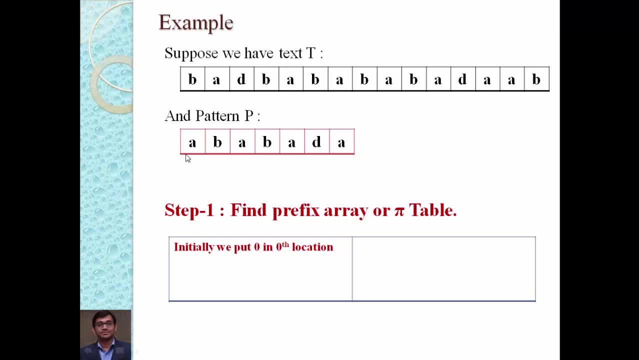 So in our pattern total seven characters are there. our first character is on 0th index, Second will be on first index, third will be on a second index, like that. So we have to put initially 0 in 0th location. So we have to just put here 0 because we have only one character. 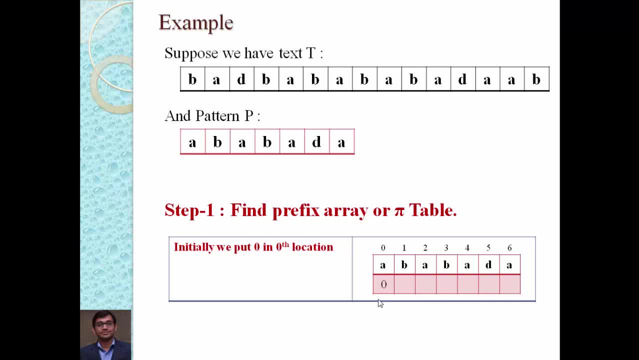 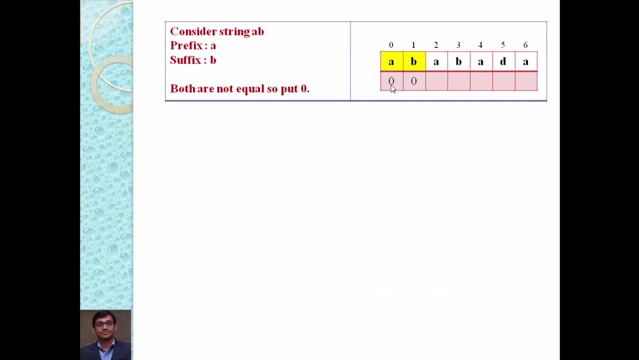 And a itself is a suffix and itself is a prefix. So only single characters are there, so that we have to put 0 here. Now our next step is we need to consider first character and second character. So we have a pair of character. Now we have a two character, a and B. 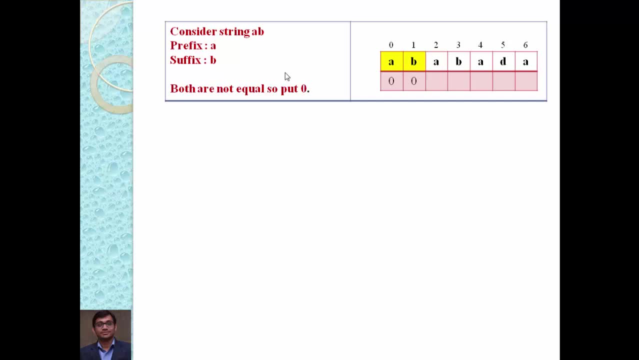 So find out all the suffix and prefix of this pair of character and B. So the prefix is a and suffix is B, because we have a two character. So the first character is a prefix and second character is suffix. Now we need to verify whether this both this: 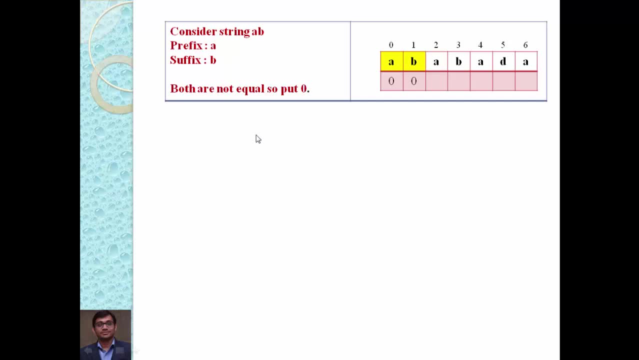 Suffix or prefix is equal or not. whenever it is equal, then we need to identify the length. But here both are not equal, so that we have to Put zero there. Now we need to consider third character. So we have a three character now in a string. That is, our a, B. 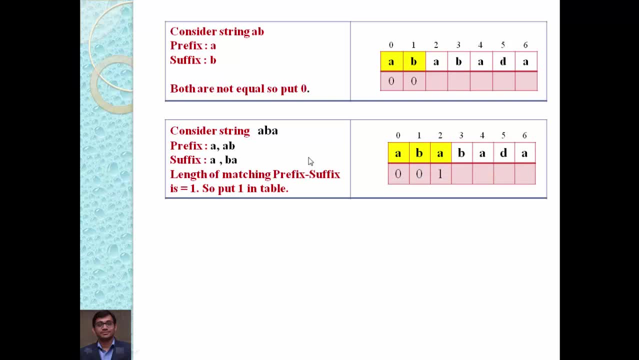 Now find out all the prefix and all the suffix. so all the prefix of a- B is a and the pair of Character that is a- B. So a is a prefix and a- B is a prefix. find out all the suffix. So a suffix means after so. 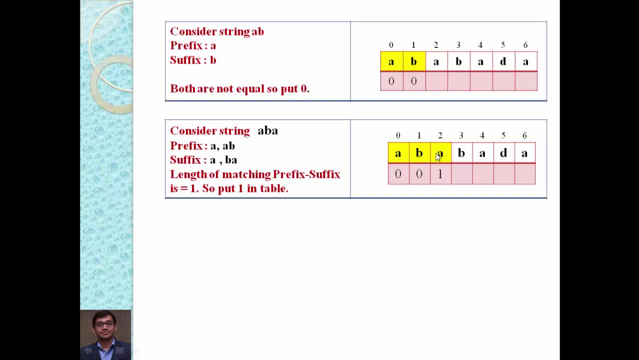 That after a we have a, two character, B and a. so the first suffix is a single character, a and Second suffix that is a pair of character B. now, from this, All the values of prefix and suffix, we need to identify The common one. so here is a common in prefix and suffix. this a B, and here is a B. 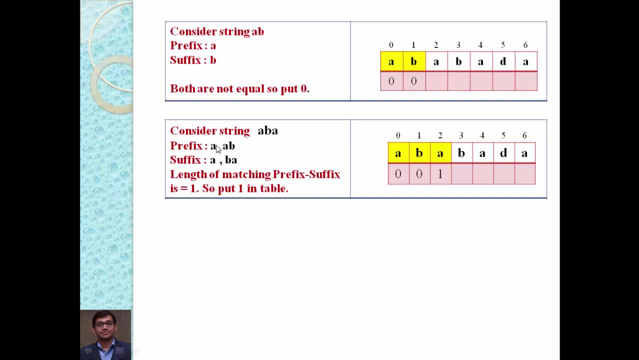 So this is not the common. so only one string is a common. that is the first. a is a prefix and A is a suffix. so the length of matching prefix suffix is equal to one, so that we need to put one here. Now we need to consider total four character, That is our a, B, a, B. 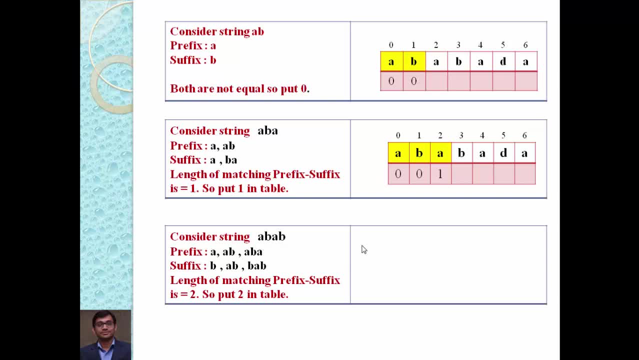 So we have now four character a, B, a, B. now find out all the prefix and suffix. So prefix means before the character. So before character B. We have a three character: a, B, a. So find out all the prefix so we can write single character a is a prefix, pair of character a, B is a prefix, and 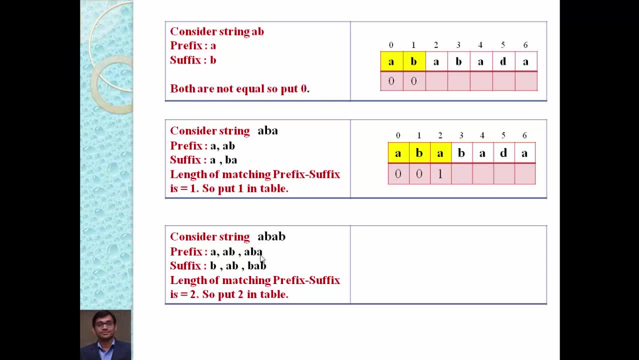 A, B, a is also prefix. find out all the suffix. So after a we have a three character B, a, B. So all the suffix is: first single character B is a suffix, then pair of- sorry- single character B is a suffix, and pair of character a- B is a suffix and a, B, a, B is also. 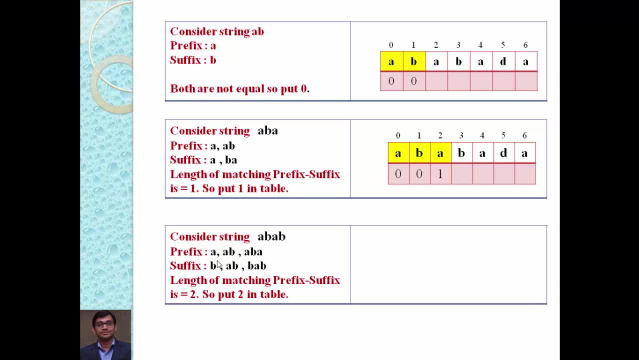 suffix. So now these are the prefix and suffix. we need to identify which one is common. So here and here B. so not common. here a and B a B and here a B. So this is the common, or it is available in both prefix and suffix. Here a, B a and this is our B a B. so it is not common. 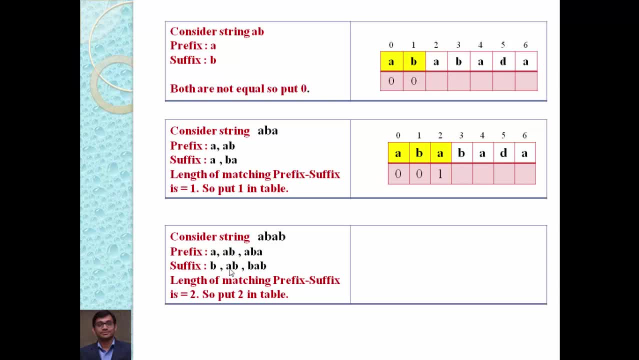 So we have our two character in prefix a- B and the suffix a- B. This: both are the equal and the length of this equal, or The common string of a prefix and suffix is equal to two, so that we need to put two there. So we have to put two here now. 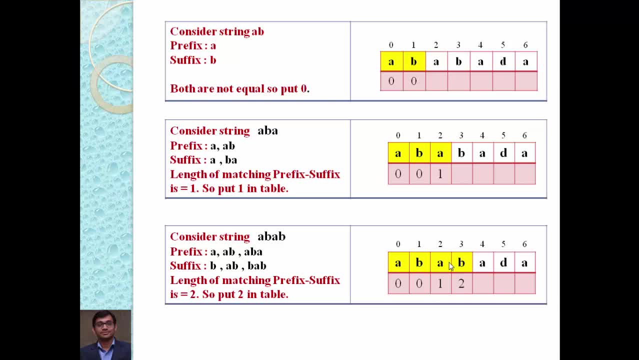 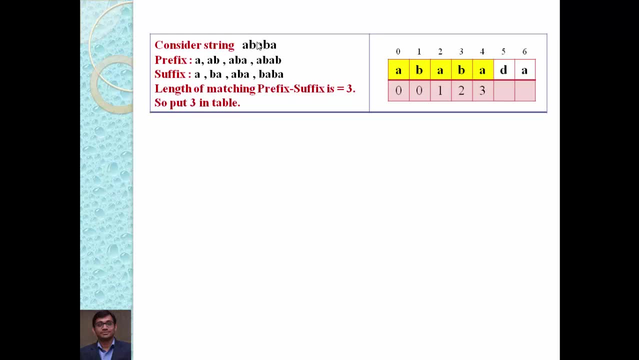 We have our different five critics: character a, B, a, B. The next one is a. so we have a total 5 different characters. So find out all the suffix. so before a we will for character a, B, a, B, and after a we have for character me, a. 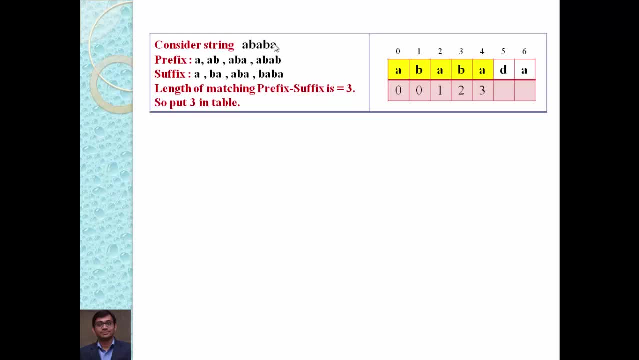 BA. So let us out first of all prefix. so before a we have a, four character: a, b, a, b. so first we need to consider first character, that is a, then after second pair is a b, third one is a b a and fourth one is a b. 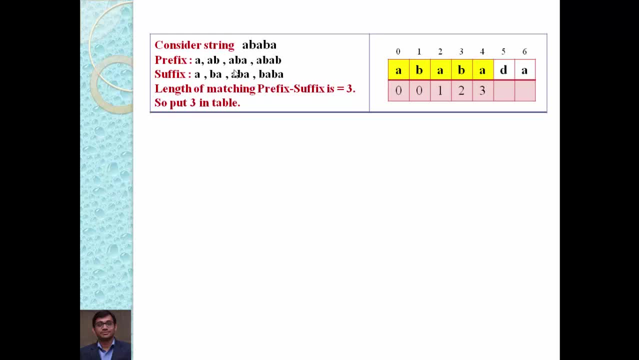 a, b. so these all are the different uh prefix. uh, now we need to identify suffix of this thing. suffix means after, so after a character we have a, b, a, b, a string. so, as per the suffix rule, we need to identify, we need to write all the suffix. so we have to start from the last character and 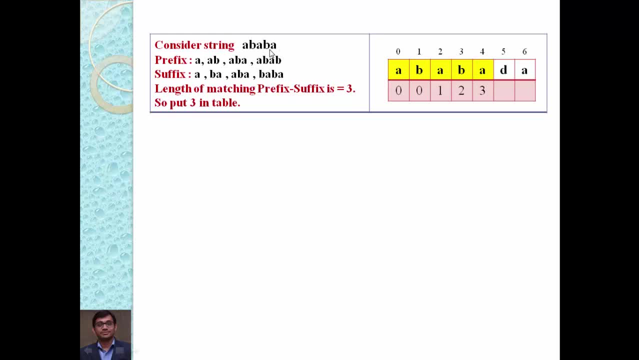 this last character is our suffix, then pair of character b a is a suffix, then a, b a is a suffix and b a, b a is also suffix. so now, out of this, all the prefix and suffix, we need to identify the common one. so a is a common in prefix and suffix. so here a, b and b a. this is not common. 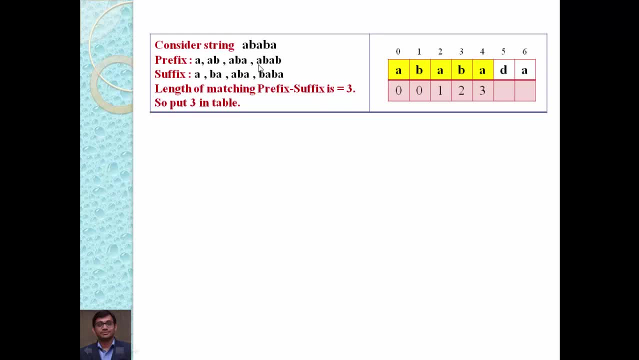 here a, b a and here a, b a is also common and these both are not the common, so we have a two pair. that is a is a common in both prefix and suffix, and this a, b, a, a, b a is common in prefix and suffix. so we need to identify, uh, the common set of character which is available in prefix as: 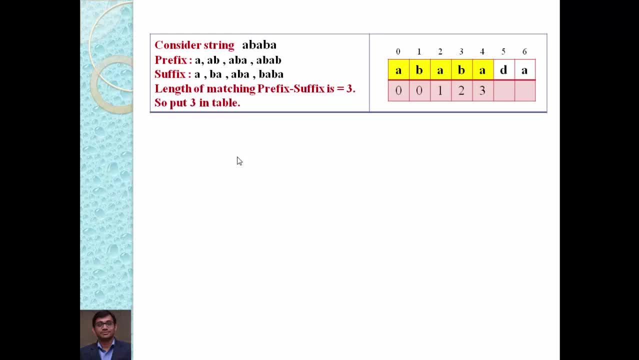 well as suffix, and which is a larger one. so among these two, this a, b, a is a larger one and has a total three different characters, so that we can say the length of the prefix and suffix is equal to three, so that we need to put three here. so just put three here. 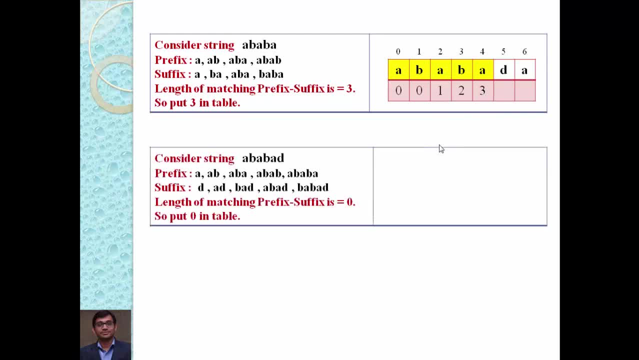 now our next character is a, d, so that we have a set of character like a, b, a, b, a, d. so find out all the prefix and suffix. so the prefix is before d. we have a set of character like a, b, a, b, a, so we can have a prefix like a single character, a, then after pair of character a, b. b, then after a, b, a, then after a, b a, b and last that is a, b a b. a same way, the suffix is we need to start from the last character, that is, a d. the first single character, d, is a suffix, then add is a suffix. b a d is a suffix. a, b a, d is a suffix and b, f, b a d is also suffix. we need to. 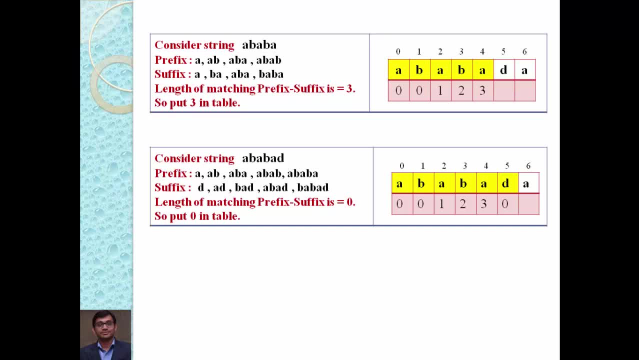 common inside the prefix and suffix. so just check: a here a, here D. not common a B, here a D is not common a B a and here B a D. not common a, B a B, here a, B a D. this is not common. here a, B a, B a and here B a, B a D. and this is also not 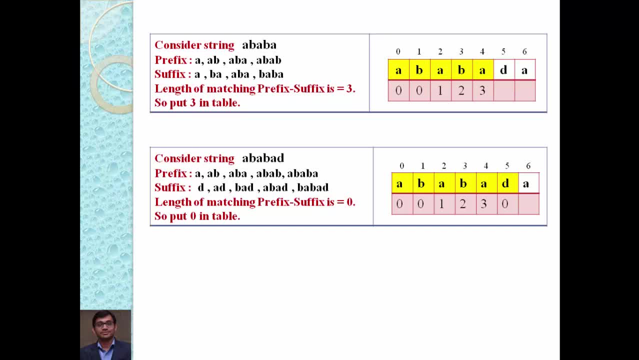 common, so that we can say the length of the matching of prefix and suffix is equal to 0, so that we need to put 0 here now the last character. so our string is a, B, a, B, a, D, a. so find out all the prefix and suffix, so all the character before. 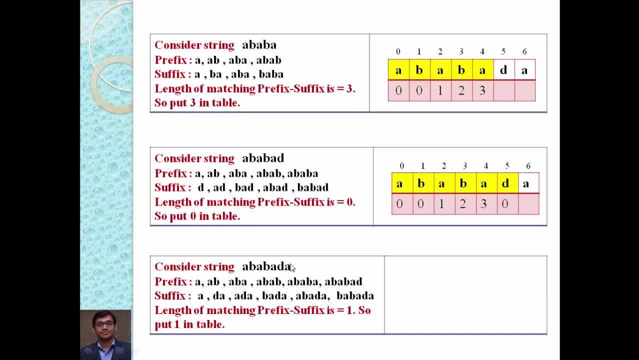 the a. so here last character is a, and before that we have a set of character like a, B, a, B, a, D, so that the single character a is a prefix, then a pair of character- a, B, is a prefix, then a, B, a is a prefix. a, B, a, B is a prefix. a, B, a, B, a is also. prefix and a, B, a, B a, D is also prefix. find out all the suffix. so after a we have a set of character like a, B, a, B, a, D, a, so that we need to start from the last character. so a is a common and we can say a is a suffix. then pair of. 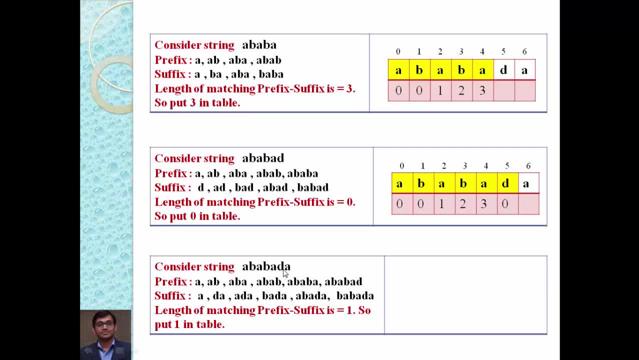 characters is a suffix. Then after ADA is a suffix, BADA is a suffix, ABADA is a suffix and BABADA is a suffix, Find out all the string of prefix and suffix and we need to identify which one is common. So A is a common in prefix and suffix AB and here DA. this is not common, Here ABA and here ADA. this is not common. Here ABAB and here BADA. this is not common. Here ABABA and here ABADA. so this is not common. 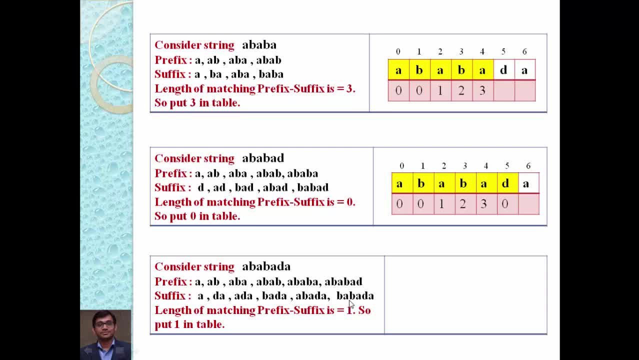 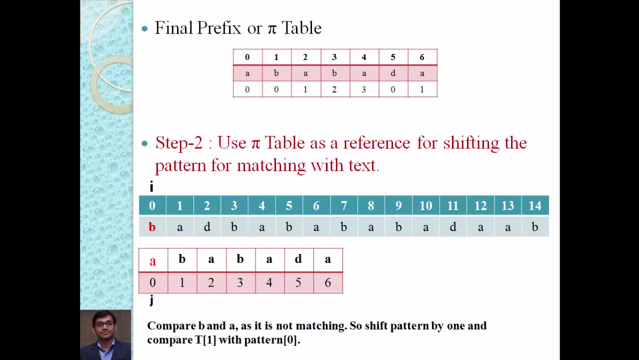 Here ABABAD, here BABADA. so these are not the common, Only one character is common, that is ABABA. Okay, so that we can say the length of matching prefix and suffix is equal to 1, so that we have to put 1 here Now. after this step, we have a final prefix or pi table. So this is the pi table, or we can say the prefix table. 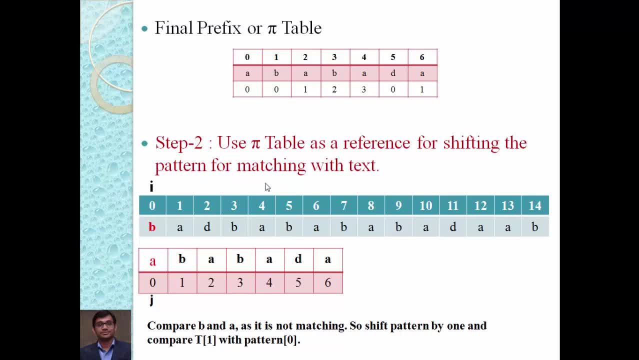 Now use this table to shift our pattern when we match our pattern with the text. So just see how we can match or how we can say the prefix table And so that we can shift our pattern with the text. So step number 2 says that use pi table as a reference for shifting the pattern, for matching with the text. 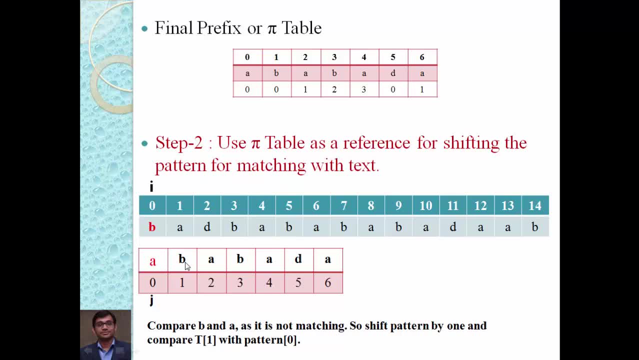 So we need to start, want to match our pattern with the text, So we need to start from the 0th index. So this is our text and this is our pattern. So let us compare our first character of text with our first character of pattern: Here it is B and here it is A, so matching is not found. 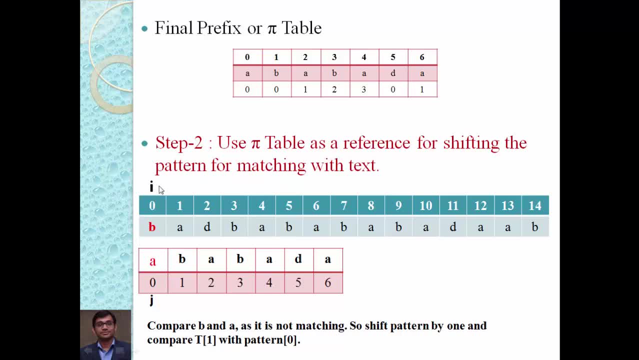 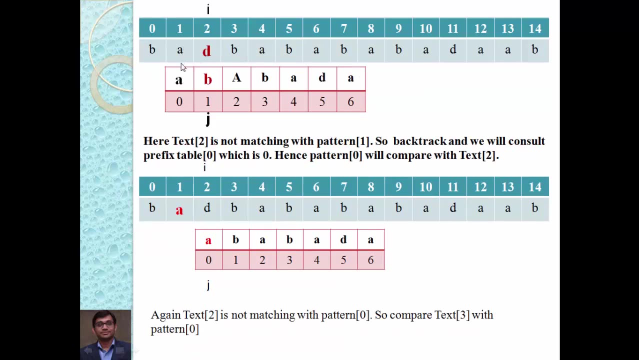 So that we need to shift 1. here I indicates the index of our tax and J indicates index of our pattern. so we need to just shift by 1. so next we will compare our a with. so both are equal. once this, both are equal, then we have to increment index I. so I will be. 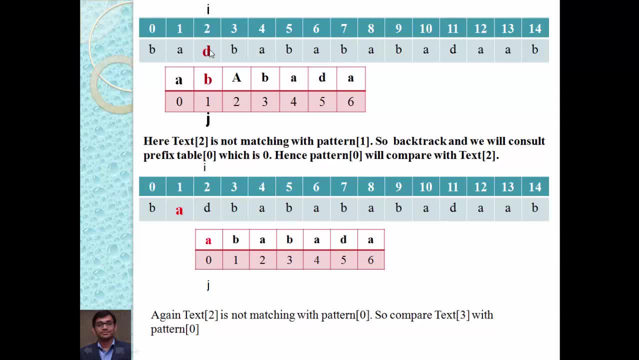 on 2 and J will be on 1. now we need to compare D and B, whether both are equal or not. so here a, B and D. both are not equal. so whenever both the characters are not equal, at the time we have to refer our a pie table and, according to: 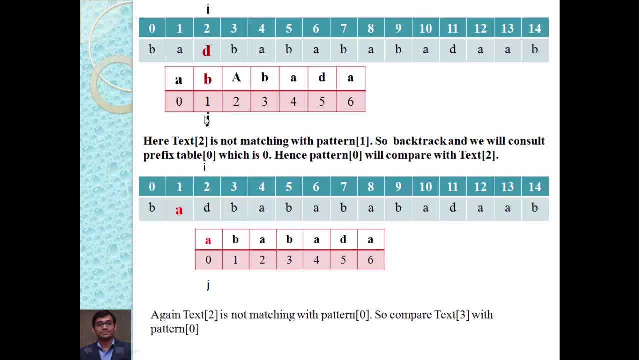 the value of pi table. we have to shift our pattern. so before that we have to perform a backtrack here on our pattern. so you have to just go back. or previous value is 0, so we need to verify the value on index 0 on our pie. 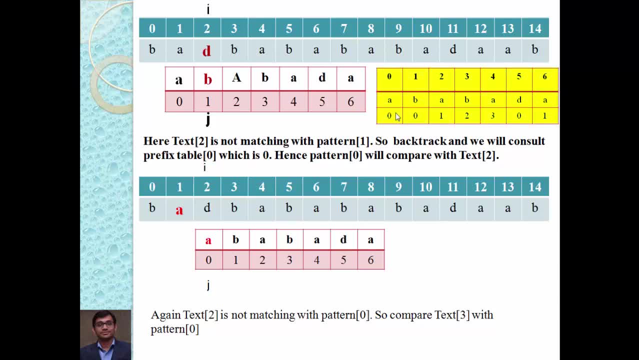 table. so this is our PI table. and on index 0 the value is 0. it indicates that we have to compare our D character, or we can say the index number 2 of our text, with 0 character or 0th index of our pattern. so we have to compare D with A again, so D. 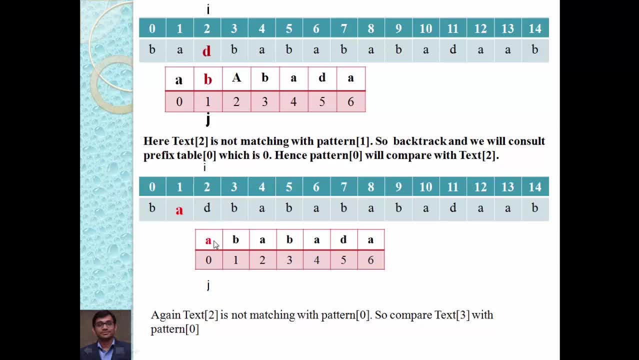 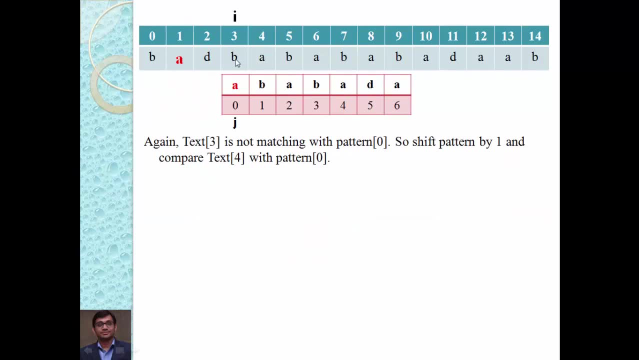 and A. both are not equal. it means that again we have to perform shift right operation. once we perform shift right operation, then we have to compare B of text with the A of pattern. so B and D, again both are not equal. so we have to perform again shift right operation, then again power of, again compare A of text. 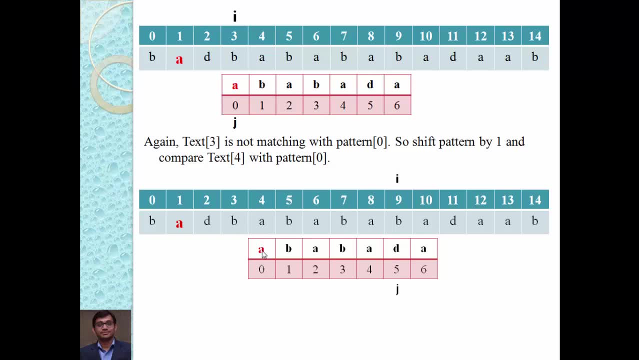 with the A of pattern. so A and A, both are the equal character. then compare next two character: B and B, both are equal. then again A and A equal, B of text and B of pattern, both are equal. the next character: A and A, both are equal. then here B and D: both are not equal. it means: 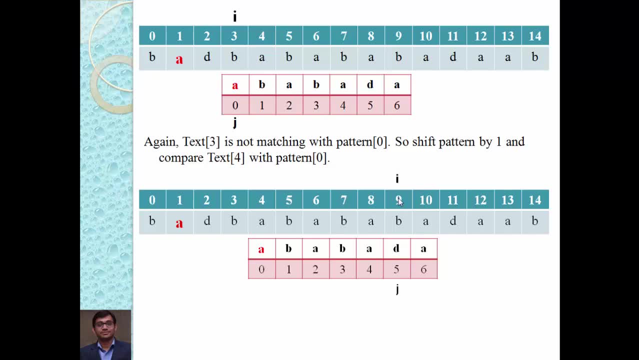 that index number 9 of our text and the value is B and index number 5 of our pattern and the value is D. both are not equal, so we have to again perform backtrack. we have to just go back. our previous value is 4, so So we have to check our pi table on index number 4.. 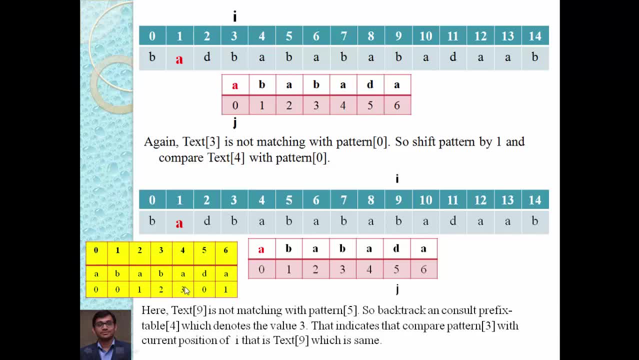 So in our pi table- this is our pi table- on index number 4- the value is 3.. It indicates that we have to compare value on third index of our pattern, that is b, with our current value of i, that is 9.. It means that b We have to compare third index of our pattern with ninth index of our text. 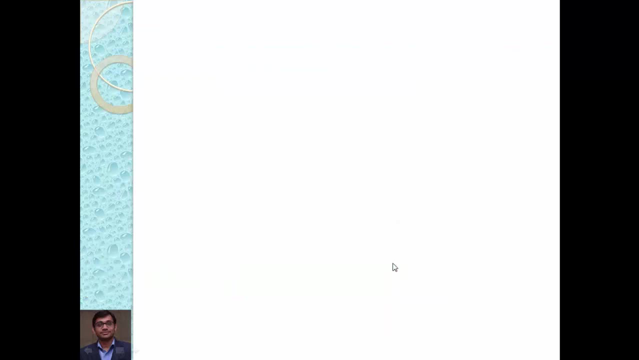 Accordingly, we have to shift our pattern, So we have to shift like that. and we have to compare ninth index of our text with third index of our pattern, So we have to compare b with b. both are equal. a- a, both are equal. d- d- both are equal. a- a, both are equal. 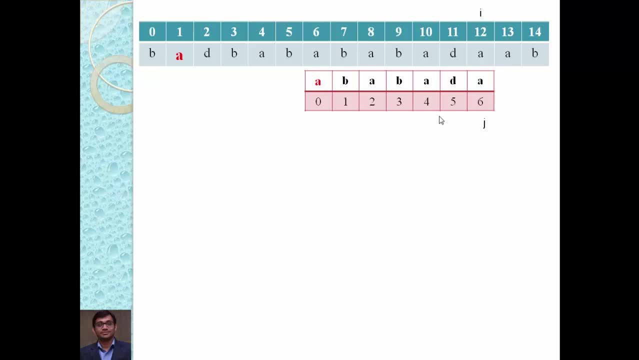 It means that all the characters are equal. It means that matching is found. Once all the characters are equal, then we have to follow our last step, that is, our step number 3.. We have one formula to identify the index and the formula is: i minus length of pattern plus 1.. 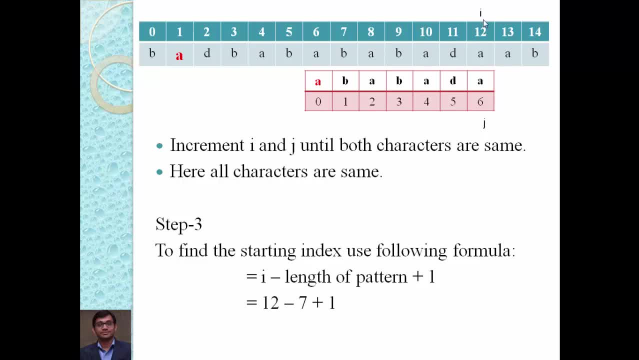 So i is equal to. currently, the last value of i is equal to 12 and the length of our pattern is equal to 7 plus 1. So that total is 6.. It means that our pattern is available inside the text on index number 6.. 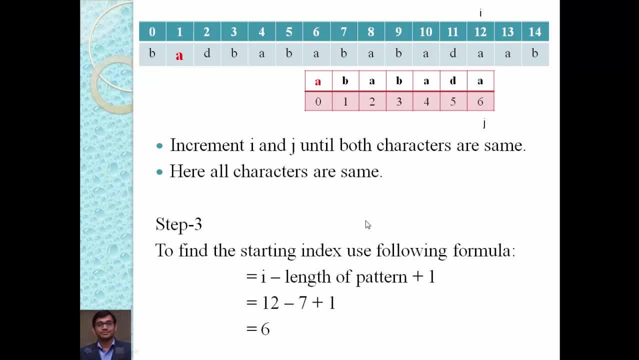 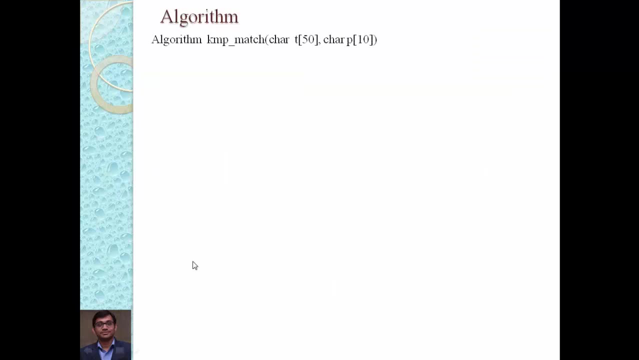 So this is the pattern which is available inside the text. So in this way we can identify whether our pattern is available in this large text or not. Now let us discuss algorithm. As per the key m p algorithm, we have to pass set of characters or we can say the text: 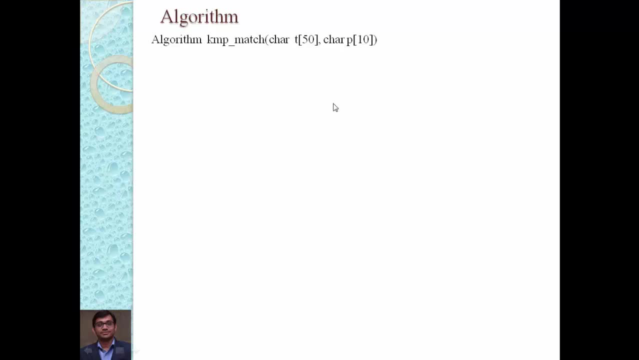 As an argument and pattern as an argument. Now we have to take one variable, and variable j is equal to 0.. First step is we need to identify length of our text, and it is suppose known as small n, Then identify length of our pattern, and it is known as, for example, m. 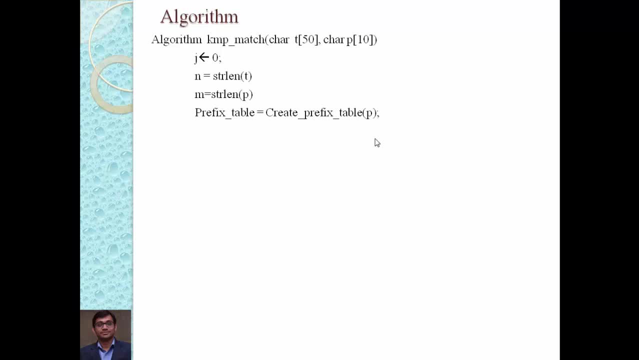 Next step is we need to generate one prefix table. as we discuss how we can generate a prefix table, So generate prefix table. Then take one of four loops, starting from: i is equal to 0 to i less than, and inside this four loop, one while loop is required to compare a character of pattern with the text, and this loop will be executed until a character of pattern and text- both are equal. 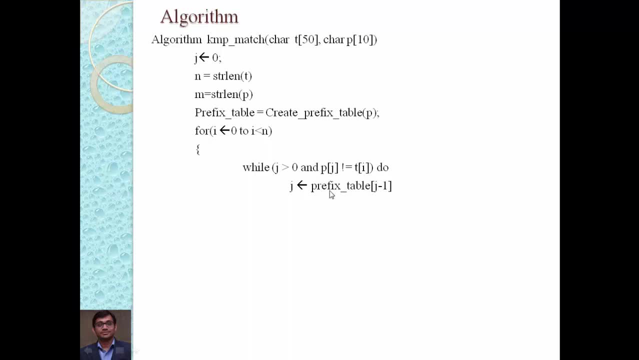 Once both are not equal, then we have to perform backtrack and we have to prefer our pi table or prefix table. Best way to do this is to use a prefix table Based on the value of a prefix table. we have to shift our pattern again. we have to compare a character of pattern with the character of text. 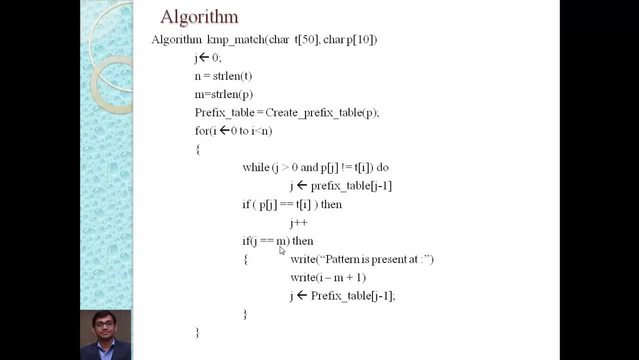 Once we reach j is equal to m. it means that once we get a whole pattern inside the text, then we have to write: a pattern is present And we have to return index number based on this formula, that is, i minus m is equal to i minus m plus 1.. 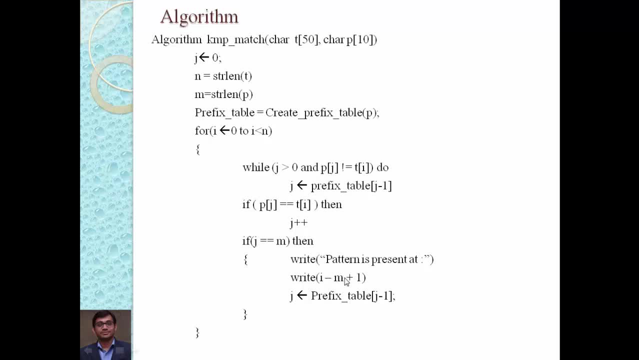 This m is nothing but the length of our pattern and i is a current index of our text and based on that we can get the index number. Then again, we have to perform, we have to refer our prefix table, we have to go back, perform backtrack and prefer our prefix table to check whether another occurrence of the pattern is available inside the text or not. 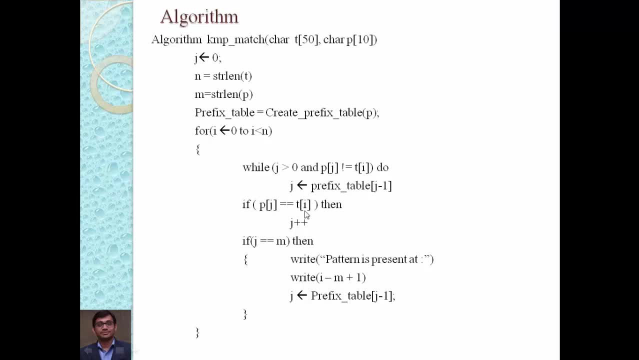 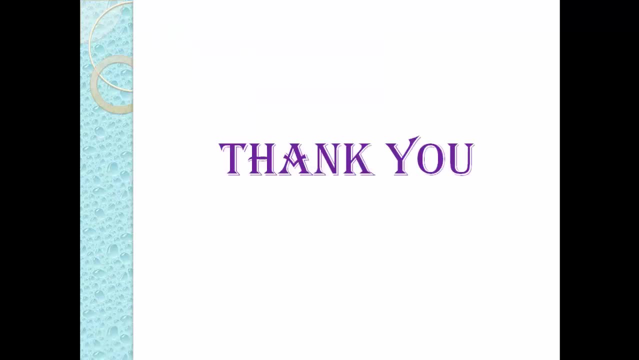 So this is all about Thank you. Thank you for watching this video.